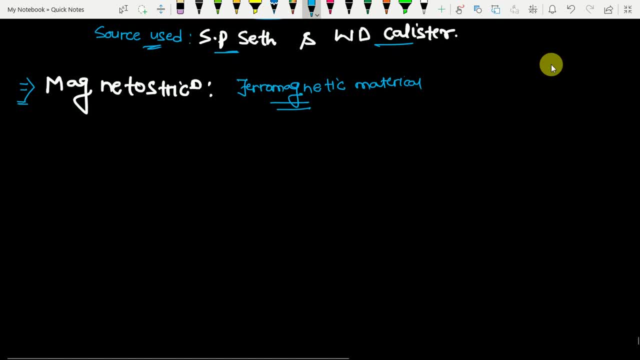 that when a ferromagnetic material is magnetized, when a ferromagnetic material, that is, when whenever a piece of specimen of ferromagnetic material is in it- is energized, there will be some change in, there will be some change in physical dimensions, physical dimensions: 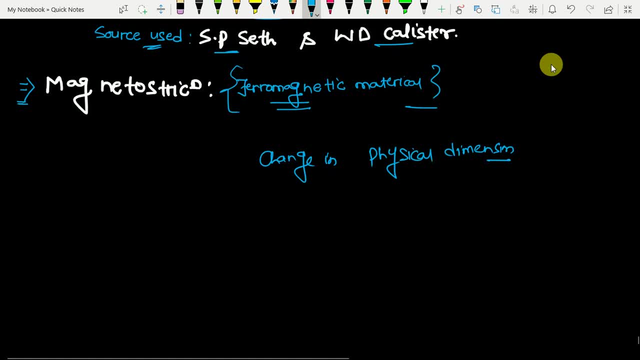 in general occur. this phenomena is known as magnet restriction- whenever we apply any extra external magnetic field, or you can say that whenever ferromagnetic material magnetized, we will observe that there will be some change in physical dimension occur. that is, there will be some change in physical dimension occur and that change in physical 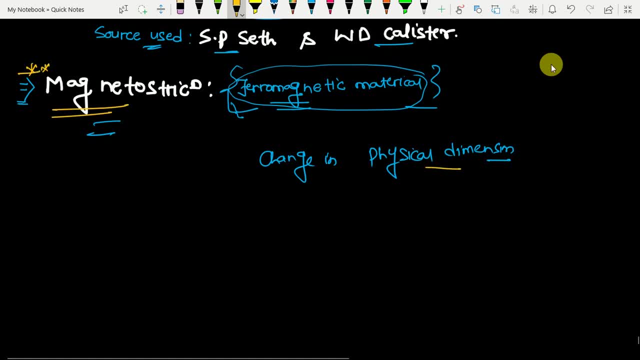 dimension is known as magnet restriction. you need to be very much concentrated for this topic because you can expect question related to this. either they will ask question in single multiple option or you can ask question, or they can ask question in a certain reason type. so we very much focused, you can expect. 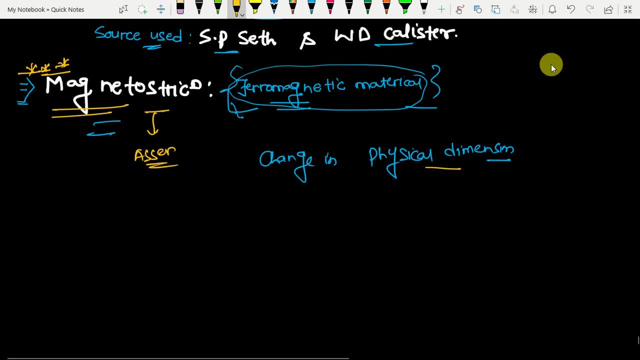 question related to these things. now there are three types of magnet magneto restrictions, types of magnetic restrictions now moving further, types of magneto restrictions. now there are three type of magnet restrictions there. these are longitudinal. longitudinal magneto restrictions, transverse, transverse magnet restrictions and third one is volume magneto restriction. 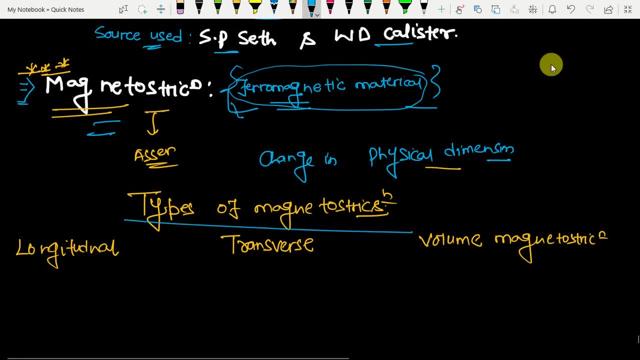 that is, there are three types of magneto strixion. types of magnet magneto strixion are longitudinal magneto strixion, transverse magneto strixion and volume magneto strixion. now you need not to be very much go in depth for these concepts. 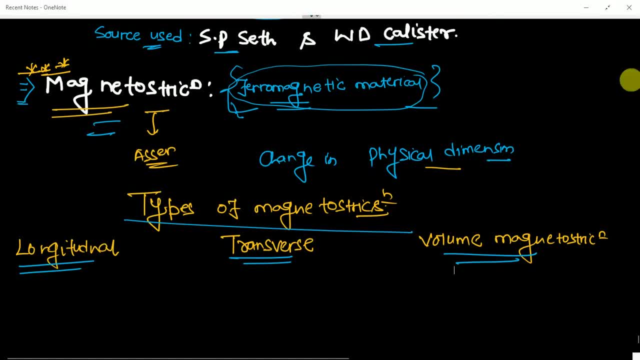 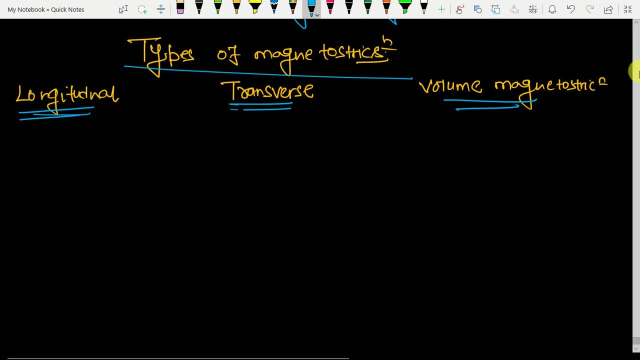 but you can know about these things we got Question can be framed from anywhere, So you need not to. you can't escape any point. So types of magneto-strictions are longitudinal, transverse and volume magneto-striction. What is longitudinal? 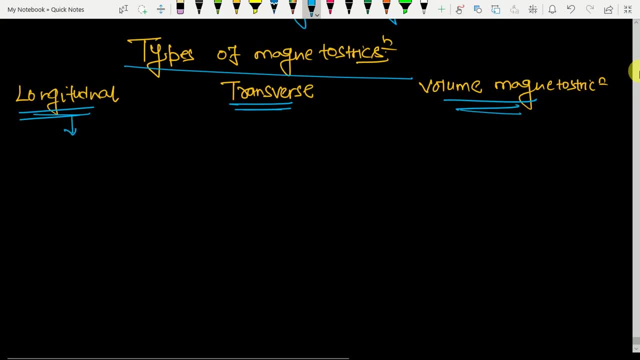 magneto-strictions. Longitudinal magneto-strictions change in length in the direction of magnetic field. That is, whenever we have applied an extra-external magnetic field to the crystal of ferromagnetic material, there will be some change in dimensions. 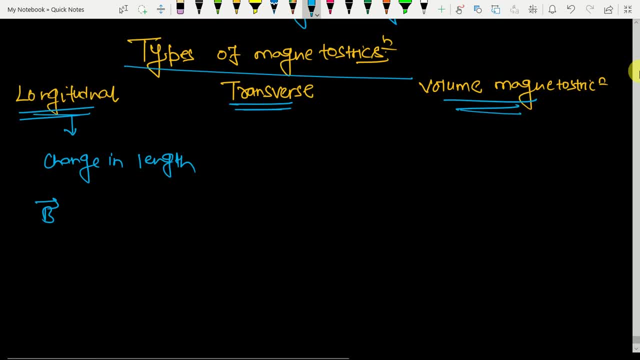 that is known as magneto-strictions. but when the change in length, that is, change in length in the direction of magnetic field, that is, when we have applied an extra magnetic field in the direction, we can expect some change in dimensions. and if the dimensional change, 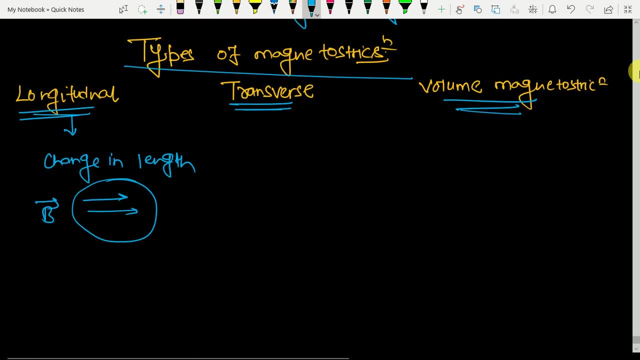 is the change in the length of that material. so you can say that that is known as longitudinal magneto-striction. This change may be increase or decrease in length. that is it. the longitudinal magnetostriction can either increase the length or decrease the length. This can cause both. 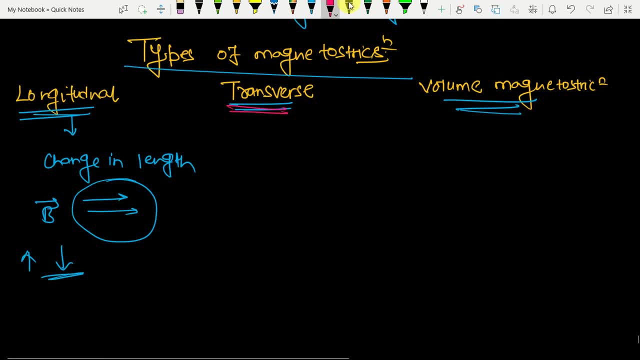 Now talking about transverse magneto-striction. transverse magneto-striction is that change in dimension perpendicular to magnetic field. in case of transverse magnetic coordination, you will this: there will be some change in dimension, but perpendicular to magnetic field and the direction of requests. 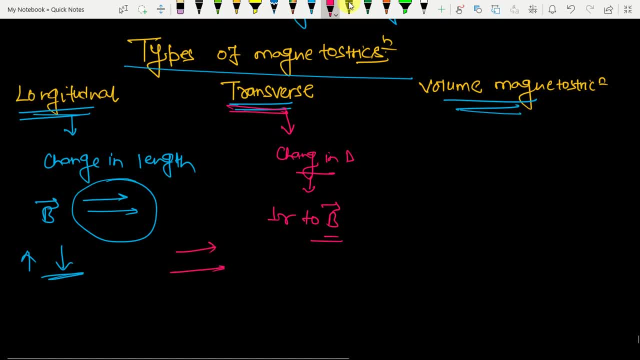 magnetic administered the direction of magnetic field. If we have applied magnetic field in this direction- the dimension of the frame- let's assume this is a ferromagnetic material- its direction will change perpendicular to the magnetic field orientation. So it's very simple. you need not to think that much. 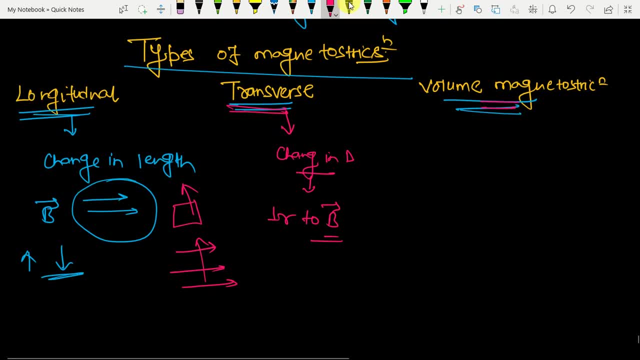 Now volume magneto-striction. What is volume magneto-striction is that change in volume resulting from the above two effects. that is when there will be some change in dimension and that in turn causes change in volume. That is known as volume magneto-striction. 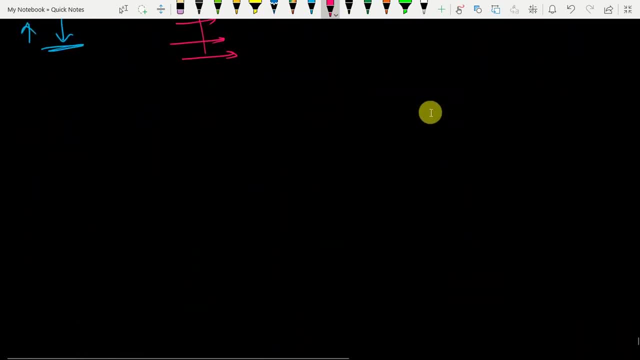 Now, this is very easy. you need not to do so much research. Just keep in mind that what is longitudinal magneto-striction, transverse magneto-striction and volume magneto-striction? Simple thing is: what will happen in longitudinal magneto-striction? 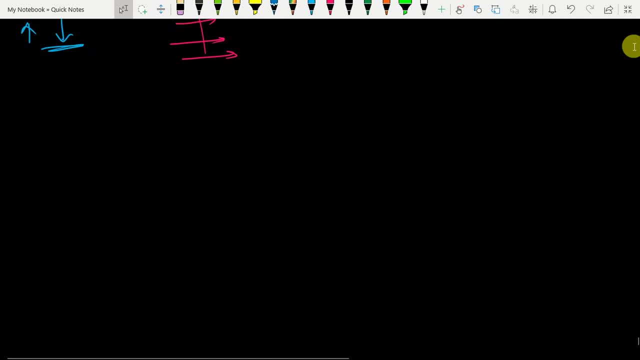 Here the change will be in length, Why? Just because we have applied some extra external magnetic field and the specimen is superimposed in extra external magnetic field, so that there will be some change in length, And this is the reason. And this is the reason. 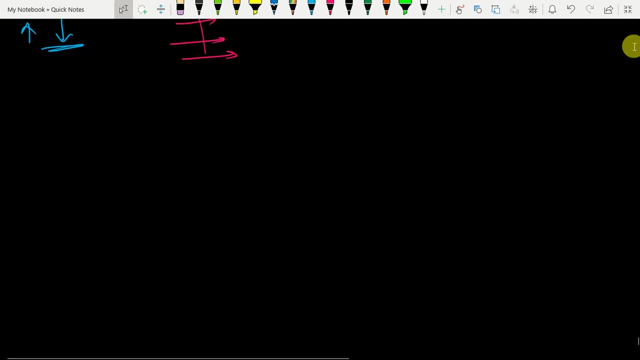 This change may be increased or decreased. Either it will increase or decrease Change in length. Now let's talk about transverse magneto-striction. What do we know about transverse magneto-striction? That there will be some change in dimension. 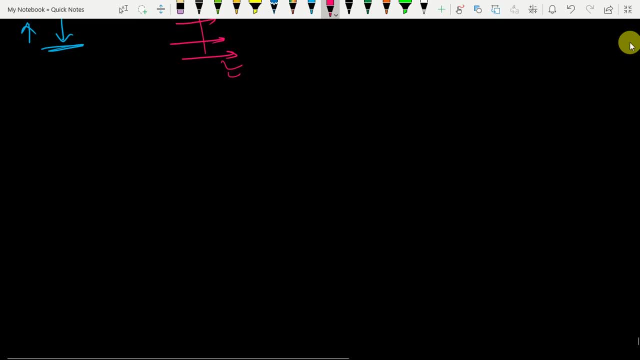 Obviously, it is a magneto-striction that will cause the change in dimensions. The dimensional change will be perpendicular to magnetic field B. That is the field which we have applied Now. third magneto-striction is volume magneto-striction. 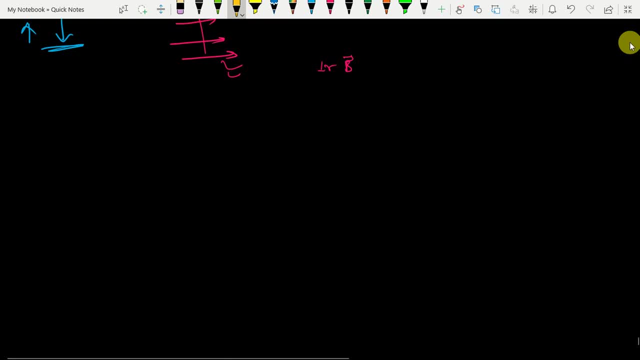 That is, change in volume resulting from the above two effects. You can say that Now the very much interesting topic is: What is the V-Lead effect? Today, each and every topic is very much important. You can expect question from each topic. 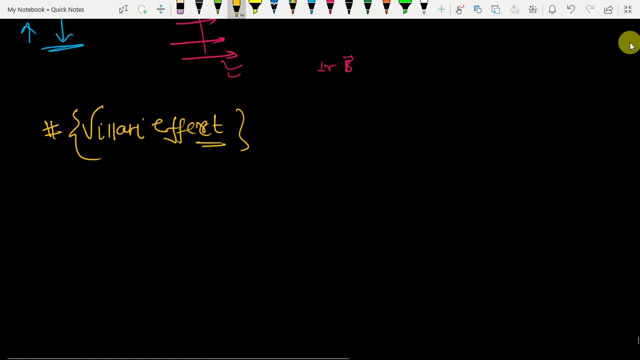 In case of engineering services examination, mainly in PREMS GS portion, Or you can say that you can expect question related to these term in either in any interview like BARC, ISRO and all. So you need to be very much focused. 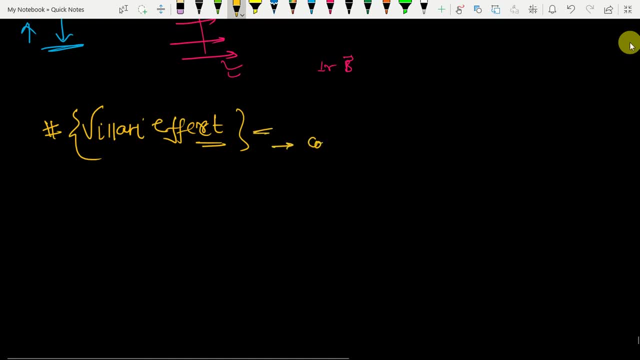 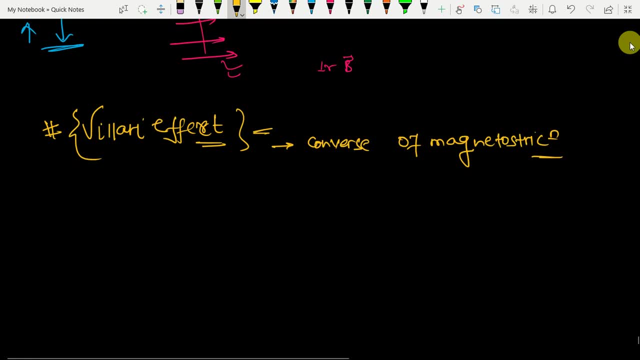 It is converse of magneto-extriction, Now how Longitudinal deformation leads to change in magnetic permeability of material in direction of applied mechanical effect. That is, there will be some longitudinal deformation, That is, change in some longitudinal dimensions leads to. 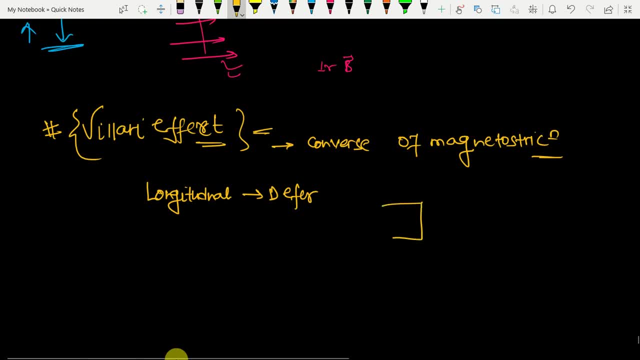 change in magnetic permeability. That is, if you have this frame and it has some longitudinal changes, then due to this there will be some change in magnetic permeability of that material. If the magnetic permeability of this material is mu1, then its change will be mu2. 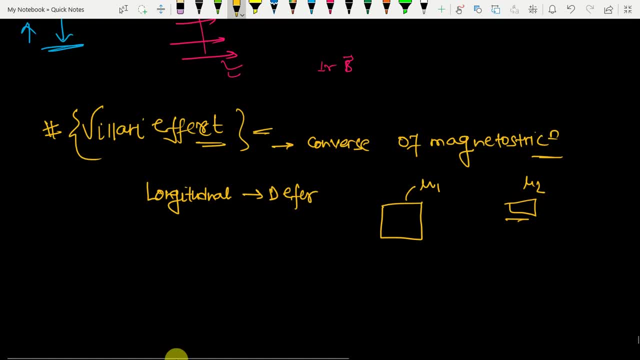 because there is some longitudinal deformation and that will in turn lead to change in magnetic permeability of that material in the direction of applied mechanical effect. That is, if we apply some mechanical effect like, let's say, stress, I have applied strain here, So there will be some change. 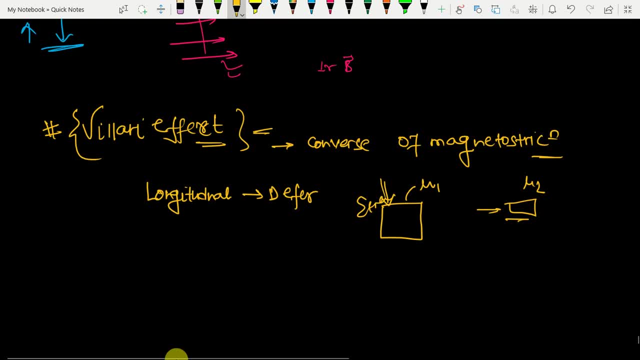 in shape and that which in turn change in magnetic permeability, That is, this will be just the reverse case of magneto-extriction. What used to happen in magneto-extriction, We put it in magnetic field and its dimensional physical features used to change. But here, 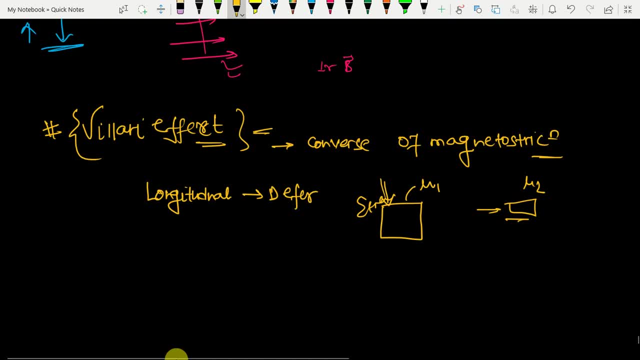 what happens in valerian effect. Valerian effect is just opposite case. We have applied some mechanical stress or mechanical strain and there will be some change in magnetic behavior like permeability of that crystal. So you can easily say that valerian effect. 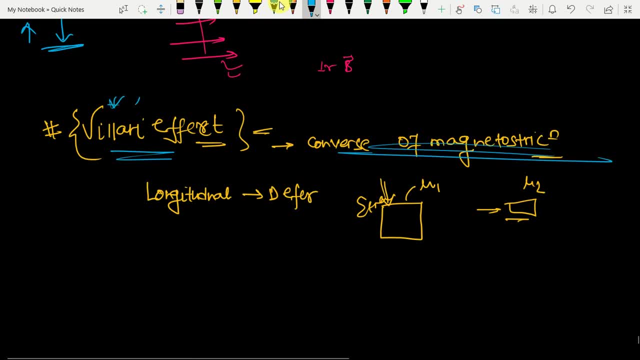 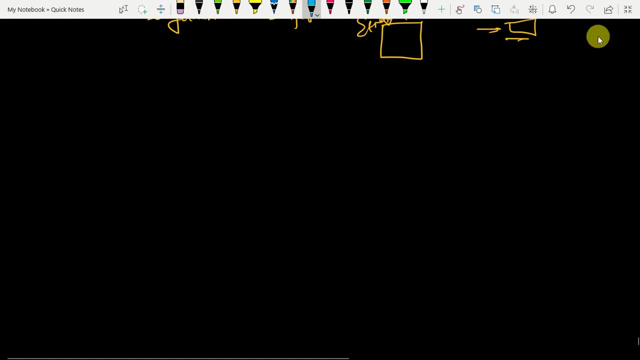 is the converse effect of magneto-extriction. It is very much important. You can expect question either in many form. Now, Moving further, application wise magnetic materials, mostly ferromagnet. We use ferromagnetic material In case of application wise in case of electrical. 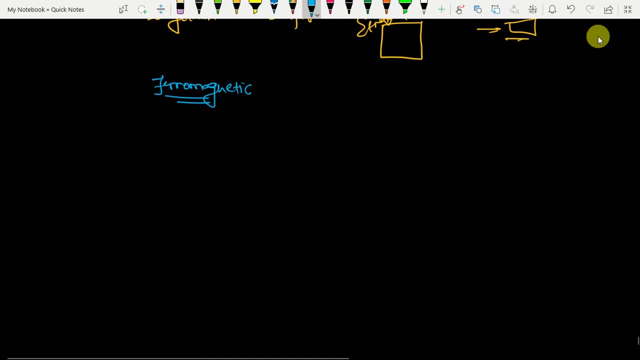 different electrical devices, like we use it in, you know, in the electrical device, like we use it in, you know, in the transformer. co we use in the three-phase, three-phase induction motor, designing of co and so many things, but we use ferromagnetic material in that case. now, mostly we use 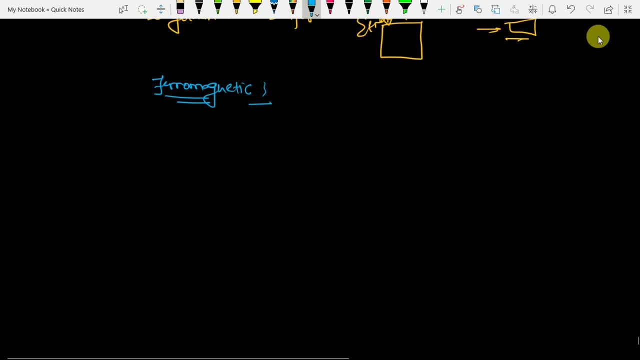 ferromagnetic material, which are used in almost all electrical devices. ferromagnetic materials are used in almost all all type of electrical devices, so you can say that ferromagnetic material is protecting layer, or you can say that ferromagnetic material is the most important. 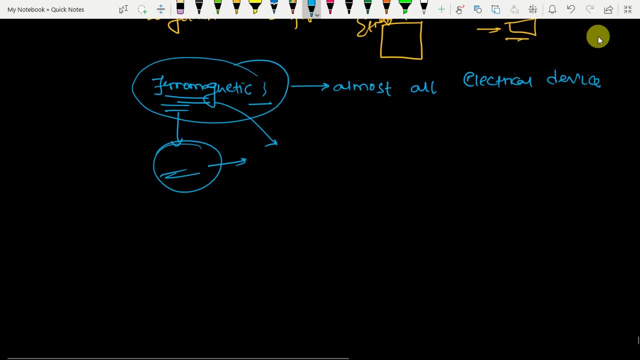 part of any electrical devices like electrical machine. either it is a static or dynamic, you can say that it is alternator or three-phase induction motor, or you can say that is a transformer. static devices- anything you ferromagnetic material is used in electrical applications. there are two type of ferromagnetic. 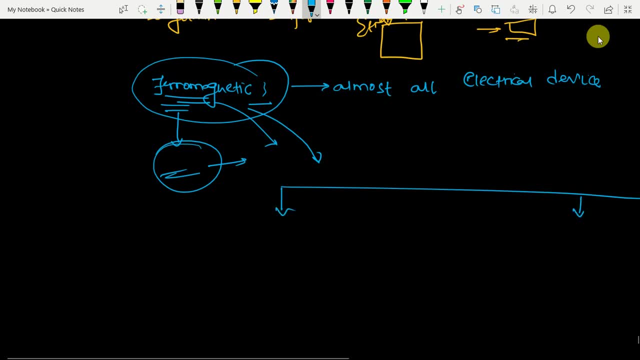 materials. there are classifying on the basis of magnetic nature. it is soft soft magnetic material and second classification is hard magnetic material. from here you can expect question in any exam for interview purpose, that is, in barc or in isro. they can ask question related to these things if you will choose subjects like 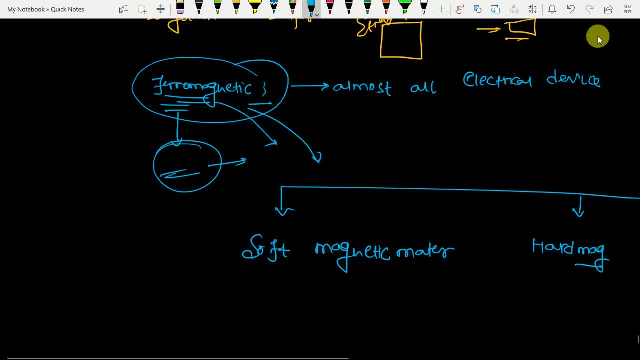 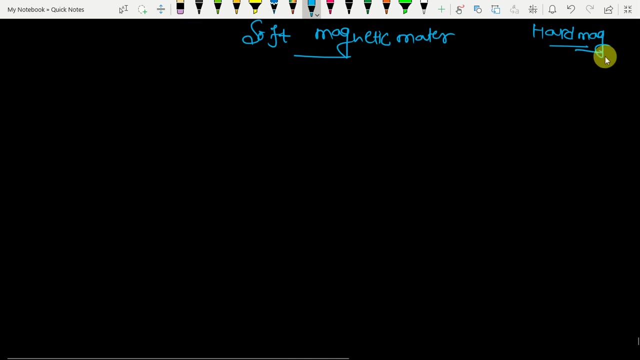 electrical machine power system for your peripheral subject. so now, soft magnetic material and hard magnetic material. let me explain you what is soft magnetic material and hard magnetic material one by one, because these are. this is very much important for for the many purpose. now i am going to explain soft magnetic material. 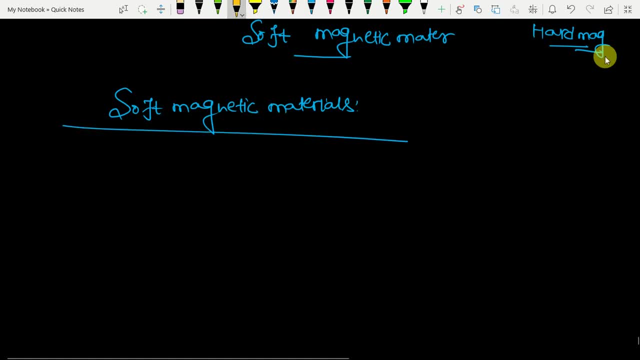 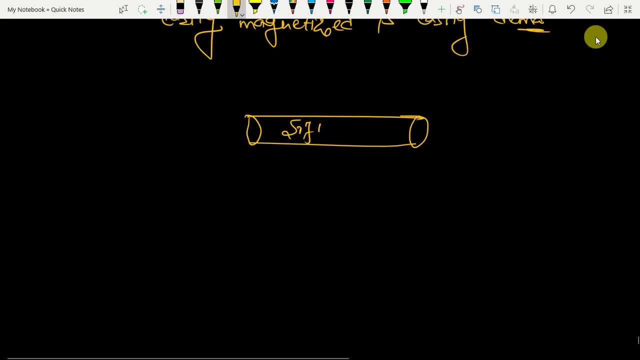 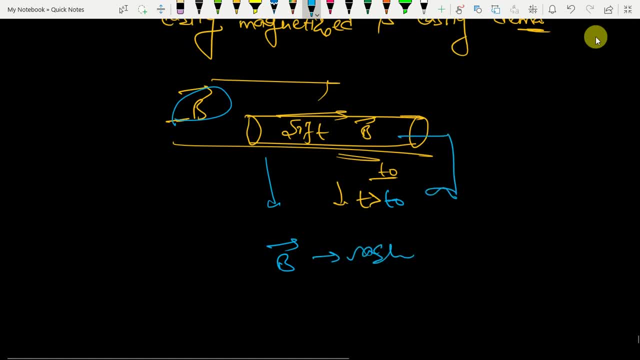 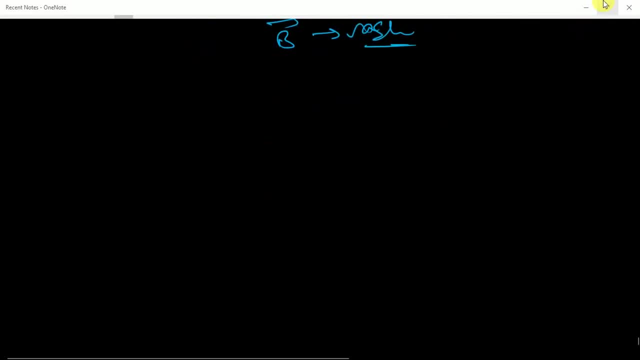 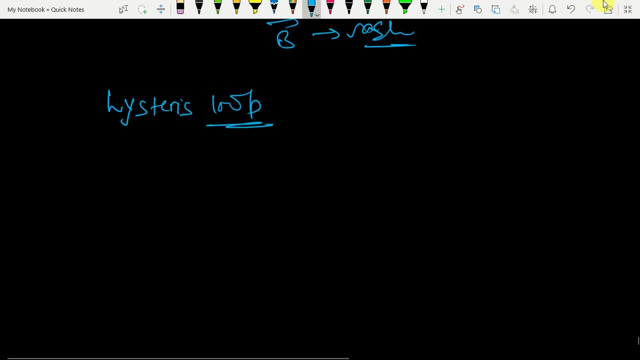 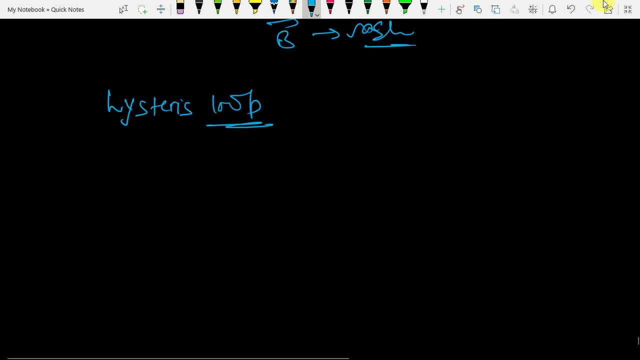 perfect for our requirement. that is, we want to design some transformer core or we want to design some any, you can say that- any alternator or any three-phase induction motor core. so you will see that there i you can justify those material through bh curve. that is how those curves 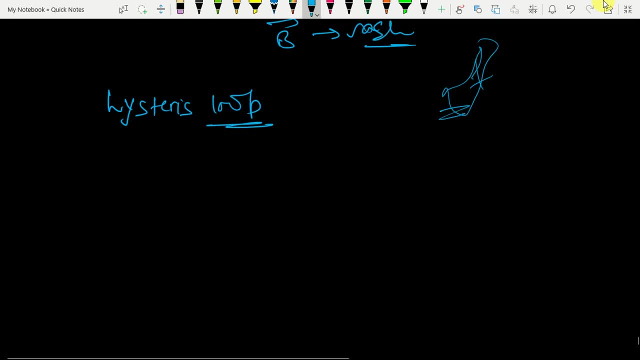 affects the or through how those curve justify the behavior or justify the characteristic of that characteristic feature of that magnetic material. so the shape of hysteresis loop in case of magnetic material has great importance in selection of that magnetic material for its application. that is, in what application we want to use that that magnetic material will be highly. 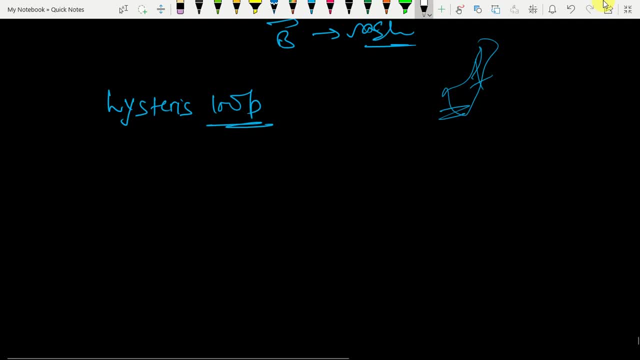 affected by the shape of that ph curve provided for that specimen or particular specimen. now, as we know that soft magnetic material, we can. we know that because we, as i have already told you, soft magnetic material will be easily magnetized as well as easily demagnetized. because what is the reason behind that reverse? 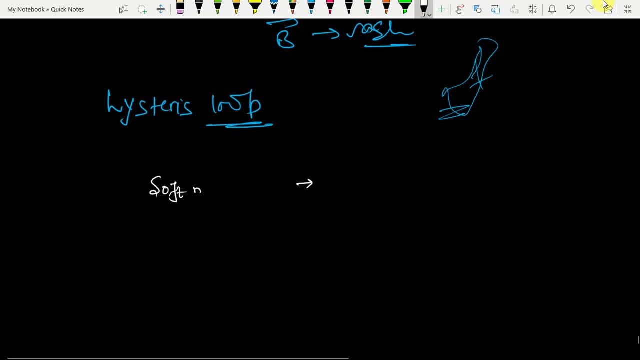 magnetization rapidly in response to alternating electric field, because there will be will be some reverse rapid magnetization. now soft magnetic material are used in construction, of course construction, of course course of transformer and ac machines. we are using soft magnetic material in case of construction or designing of of transformer core and ac. 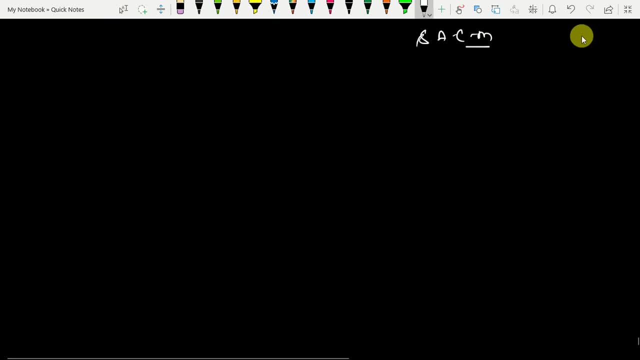 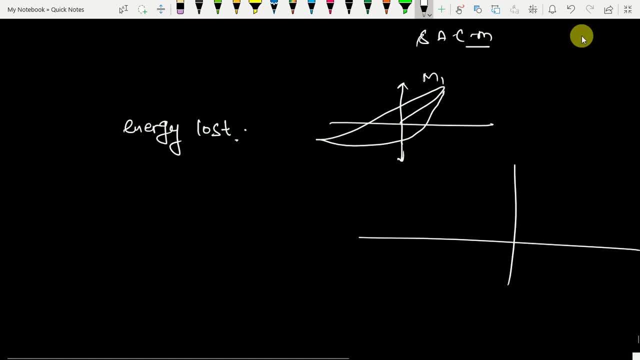 let's say material one, material one, this hysteresis curve. let's say material one, material one, this hysteresis curve. let's let me design you material two, hysteresis curve. let's let me design you material two, hysteresis curve. 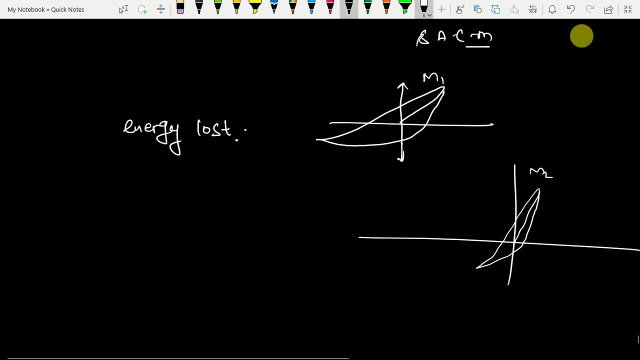 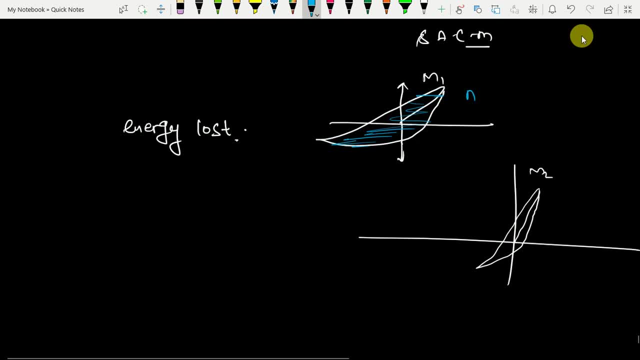 the area. you can say that the area. you can say that the area here, the area here, the area here. its bh curve area more, its bh curve area more, its bh curve area more and its bh curve area less a2 and its bh curve area less a2. 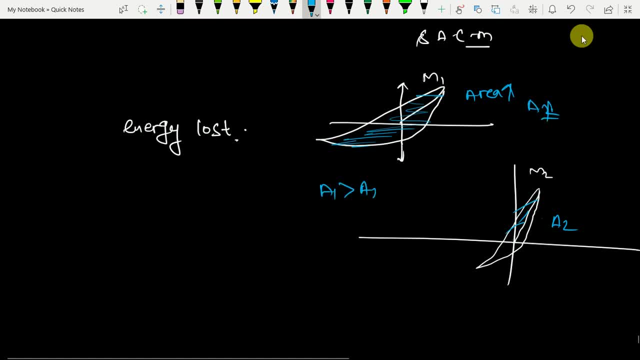 and its bh curve area less a2: save, even, even, save, even, even save, even even a1 is greater than a2. so from this you: a1 is greater than a2. so from this you: a1 is greater than a2. so from this you can conclude that a1 will have much. 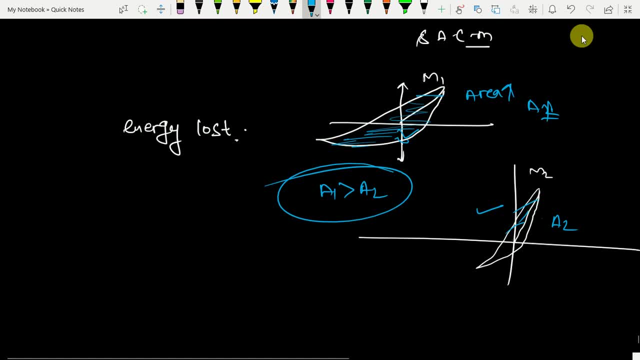 can conclude that a1 will have much. can conclude that a1 will have much more energy dissipation as compared to a2. more energy dissipation as compared to a2. more energy dissipation as compared to a2. either it is in form of, either it is in form of. 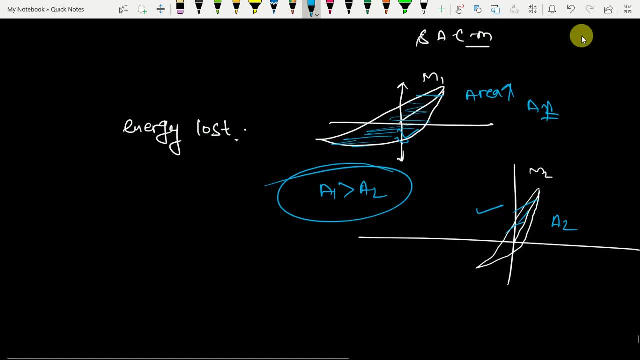 either it is in form of eddy current or hysteresis loss, so be eddy current or hysteresis loss. so be eddy current or hysteresis loss. so be very much careful. you can very much careful, you can very much careful. you can judge any uh ferromagnetic material or 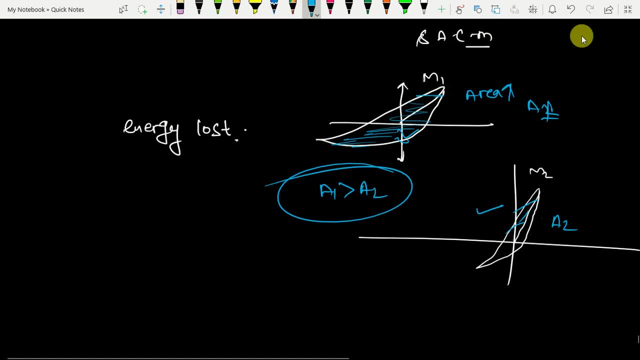 judge any uh ferromagnetic material. or judge any uh ferromagnetic material or soft magnetic material through their soft magnetic material, through their soft magnetic material, through their characteristic bh curve that is characteristic bh curve. that is characteristic bh curve that is lagging of p by h ratio. now, 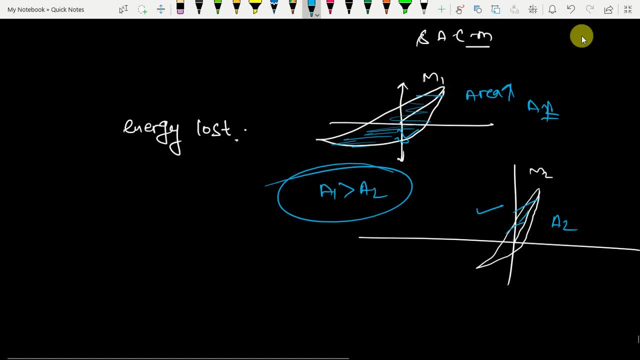 materials having small hysteresis losses, materials having small hysteresis losses, materials having small hysteresis losses, are soft magnetic materials. we are very are soft magnetic materials. we are very are soft magnetic materials. we are very much known about these things, that is. 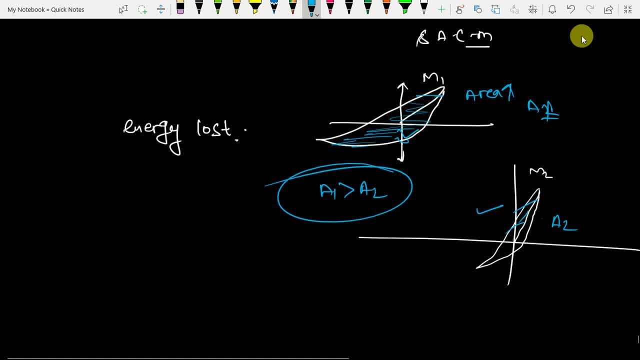 much known about these things. that is much known about these things. that is, the area curve means the area of the ph. the area curve means the area of the ph. the area curve means the area of the ph. curve, curve, curve accommodations: come then it. it can be. 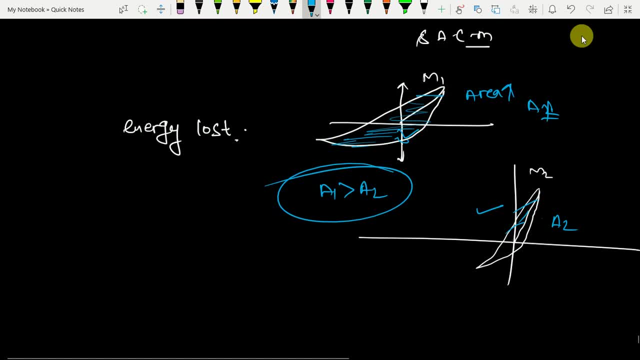 accommodations. come then it. it can be accommodations. come then it. it can be easily. we can easily say that this this easily, we can easily say that this this easily. we can easily say that this, this material will be material, will be material, will be very efficient for us and it will give. 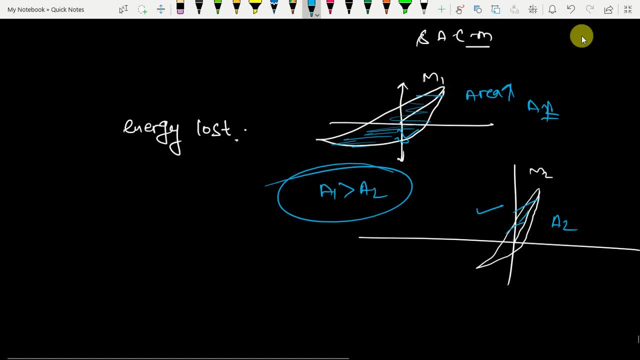 very efficient for us and it will give very efficient for us and it will give higher efficiency because the energy loss higher efficiency, because the energy loss higher efficiency, because the energy loss will be less will be less will be less. now high permeability and high saturation. now high permeability and high saturation. 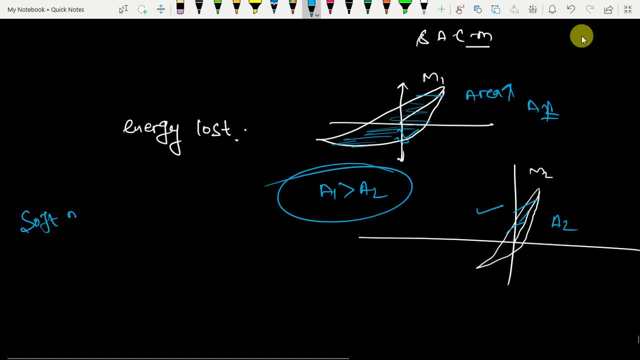 now high permeability and high saturation. magnetization in case of soft magnetic magnetization. in case of soft magnetic magnetization, in case of soft magnetic material, material, material, it has features. first thing will be it has features, first thing will be it has features. first thing will be energy loss. come over that energy loss. 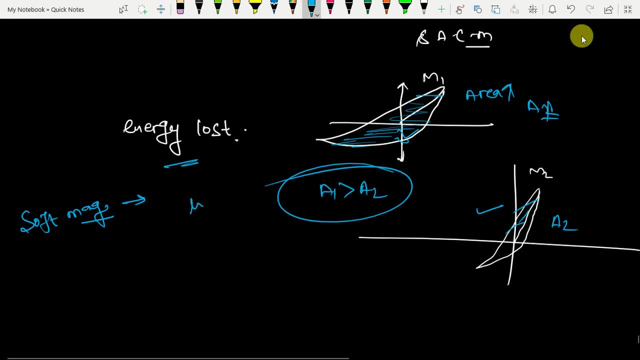 energy loss: come over that energy loss. energy loss: come over that energy loss will be less. second point will be: will be less. second point will be: will be less. second point will be: permeability high the permeability will permeability high the permeability will permeability high, the permeability will be high. that is acceptance of magnetic. 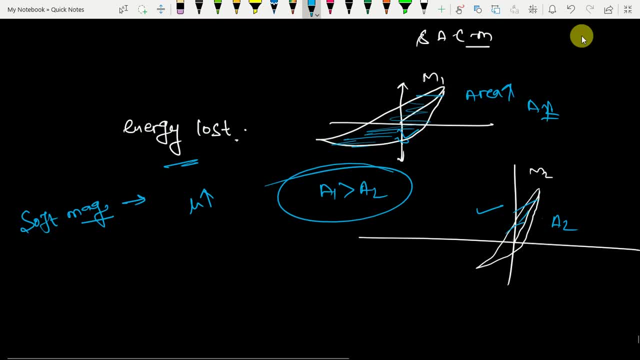 be high. that is acceptance of magnetic be high, that is acceptance of magnetic lines of forces- will be high. lines of forces will be high. lines of forces will be high. and saturation, magnetization and saturation: magnetization and saturation, magnetization: m. saturation. saturation. magnetization is m. saturation, saturation, magnetization is: 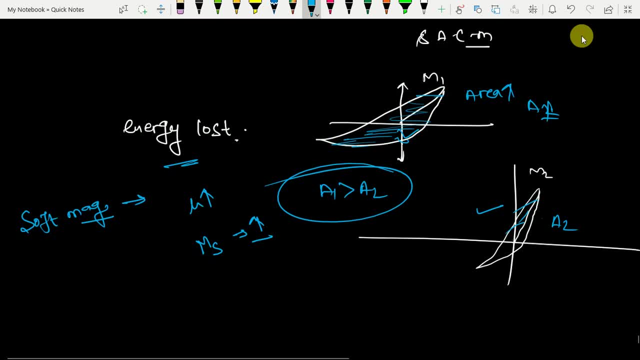 m saturation. saturation, magnetization is high, high, high. that is the transformer core or the core. that is the transformer core or the core. that is the transformer core or the core, or the material that we are using for, or the material that we are using for, or the material that we are using for making of transformer core or ac machines. 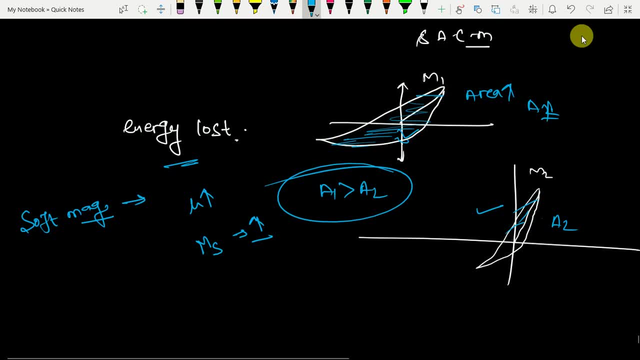 making of transformer core or ac machines. making of transformer core or ac machines. will we have high magnetic saturation? will we have high magnetic saturation? will we have high magnetic saturation level? that is, the machine will not level. that is, the machine will not level. that is, the machine will not saturate easily. simple. 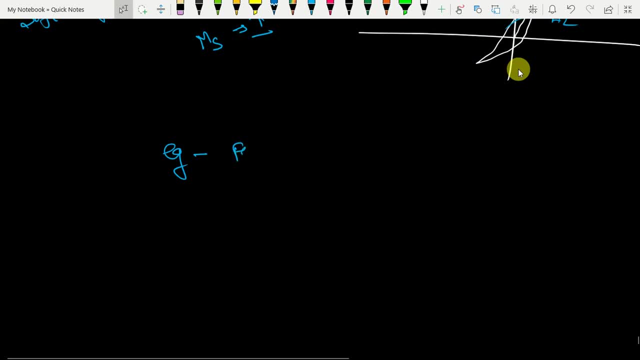 saturate easily, simple. saturate easily simple. now example: let's say iron silicon. now example. let's say iron silicon. now example: let's say iron silicon alloy. in this case, five percent of alloy. in this case, five percent of alloy. in this case, five percent of silicon is added. silicon is added. silicon is added. iron nickel alloy. iron nickel alloy- iron nickel alloy- in this case, 36 percent of nickel is. in this case, 36 percent of nickel is. in this case, 36 percent of nickel is added. added. added example: also is ferrite. example: also is ferrite. 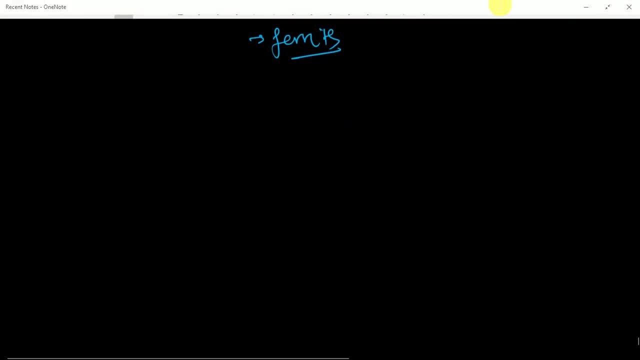 example also is ferrite. ferrites is also soft magnetic material. ferrites is also soft magnetic material. ferrites is also soft magnetic material, now moving forward and knowing the hard, now moving forward and knowing the hard now moving forward and knowing the hard magnetic material now moving forward and knowing the hard magnetic material. 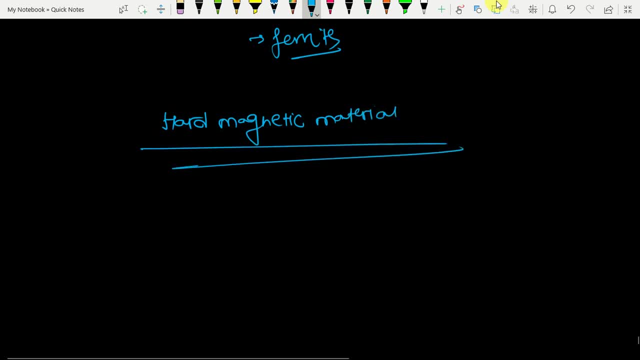 now moving forward and knowing the hard magnetic material. now the second classification is hard. now the second classification is hard. now the second classification is hard magnetic material. so you can say that: what magnetic material? so you can say that, what magnetic material. so you can say that: what do you mean by the term hard magnetic? 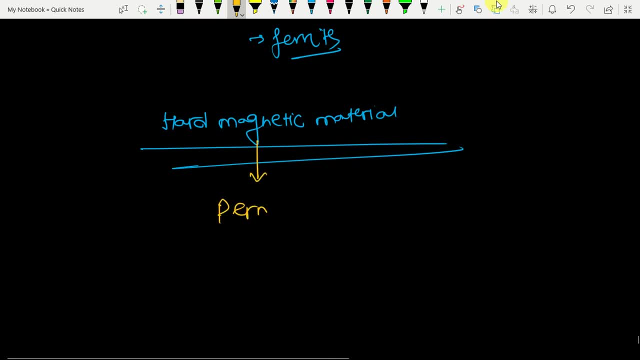 do you mean by the term hard magnetic? do you mean by the term hard magnetic material? hard magnetic material? we call material hard magnetic material. we call material hard magnetic material. we call permanent permanent magnets. these hard permanent magnets, these hard permanent magnets, these hard magnetic materials is known as permanent. 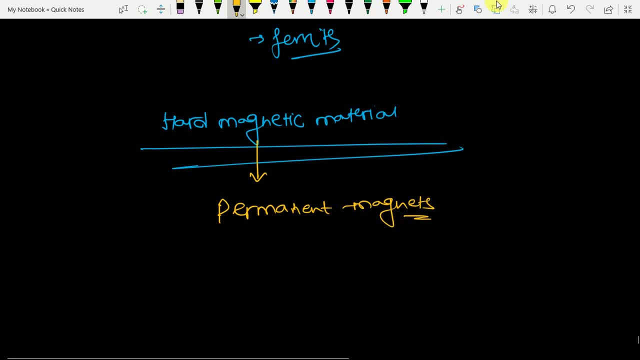 magnetic materials is known as permanent magnetic materials, is known as permanent magnets. now these materials are magnets. now these materials are magnets. now these materials are difficult to demagnetize. they retain, difficult to demagnetize. they retain difficult to demagnetize. they retain magnetism even after removal of film. 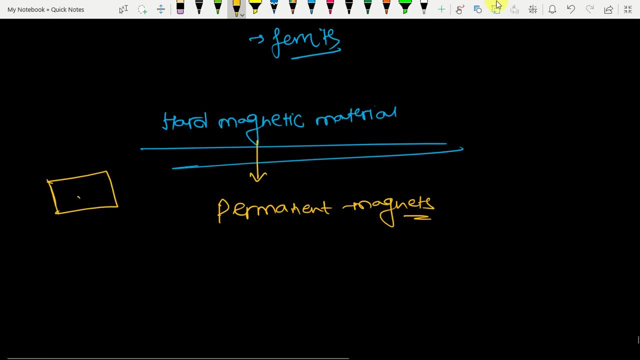 magnetism even after removal of film. magnetism even after removal of film, that is let's take. i have taken a that is let's take. i have taken a that is let's take. i have taken a specimen of hard magnetic material, say. specimen of hard magnetic material, say: 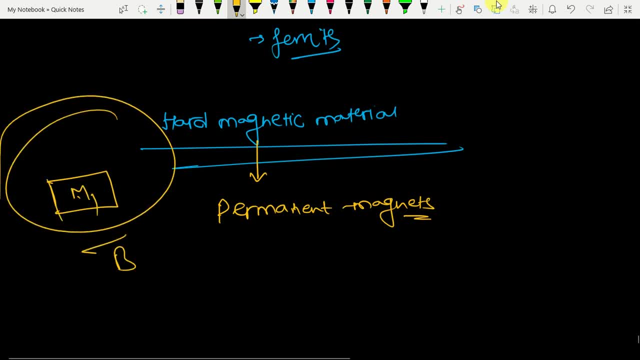 specimen of hard magnetic material, say m1, and we have provided an extra m1, and we have provided an extra m1 and we have provided an extra external magnetic field b, external magnetic field b, external magnetic field b- and it achieves some magnetic intensity and it achieves some magnetic intensity. 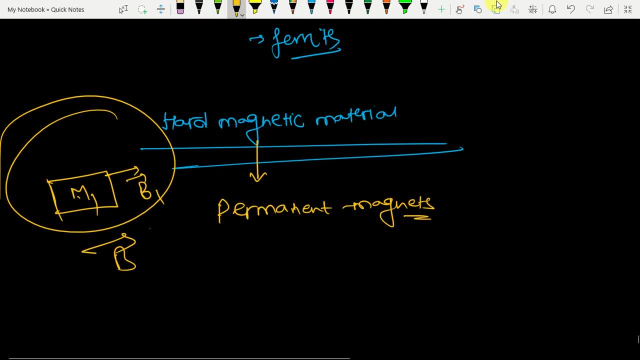 and it achieves some magnetic intensity. or magnetization- this, that is b1. or magnetization- this, that is b1. or magnetization this, that is b1. after removal of this magnetic field, the. after removal of this magnetic field, the. after removal of this magnetic field, the hard magnetic material will retain its. 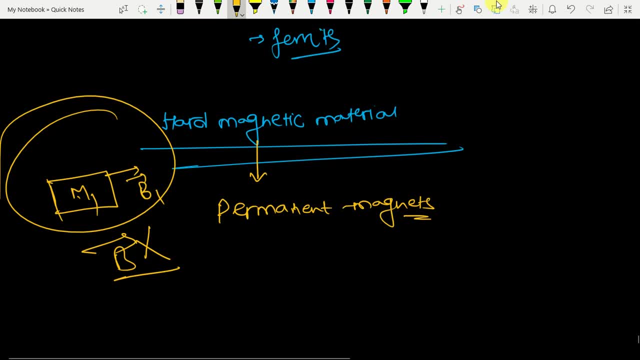 hard magnetic material will retain its hard magnetic material will retain its property of magnetization and it's not property of magnetization and it's not property of magnetization. and it's not very easy to remove that. very easy to remove that, very easy to remove that residual magnetism which is just 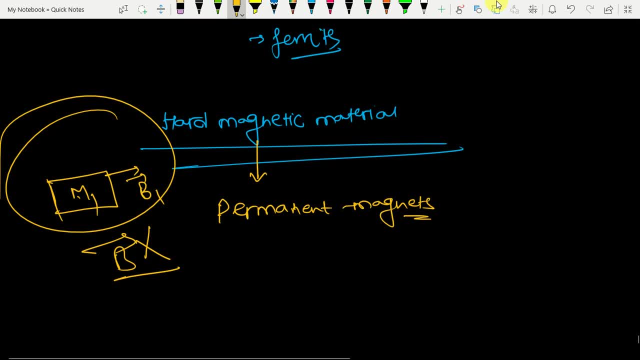 residual magnetism, which is just residual magnetism, which is just consigned inside that magnetic material, consigned inside that magnetic material, consigned inside that magnetic material. that is hard magnetic material. so you, that is hard magnetic material, so you, that is hard magnetic material. so you can say that it is very difficult in 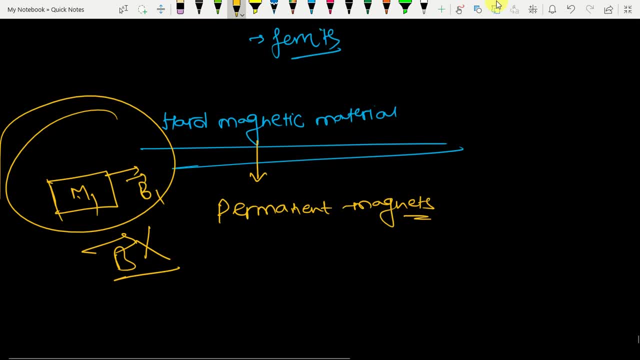 can say that it is very difficult. in can say that it is very difficult in case of hard magnetic materials, to case of hard magnetic materials, to case of hard magnetic materials, to remove or to demagnetize or to retain: remove or to demagnetize or to retain. 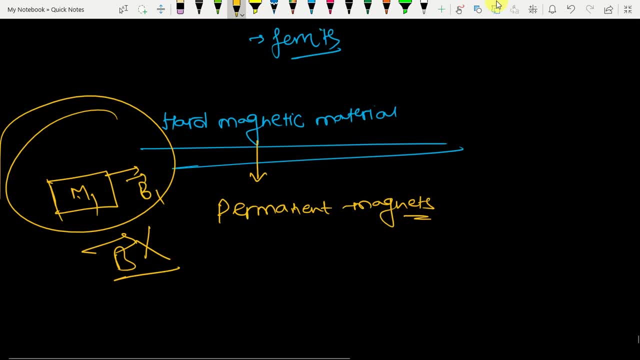 remove or to demagnetize or to retain their, their, their non-magnetic properties, which they are non-magnetic properties, which they are non-magnetic properties, which they are achieving or which they have achieving or which they have achieving or which they have framed before. so you can say that 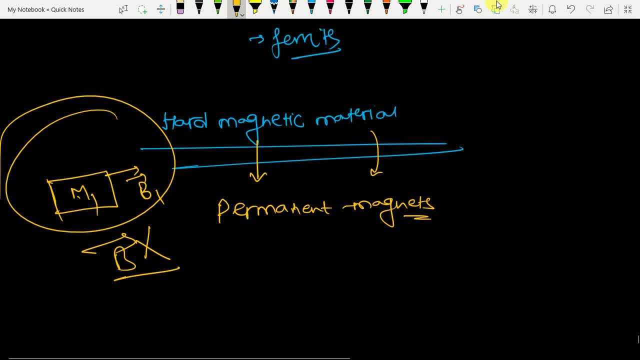 framed before, so you can say that framed before, so you can say that that's why hard magnetic material are. that's why hard magnetic material are. that's why hard magnetic material are used to making permanent magnets. used to making permanent magnets. used to making permanent magnets. it will retain having some retentivities. 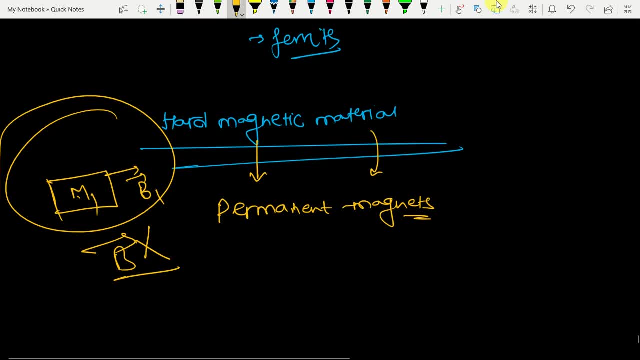 it will retain having some retentivities. it will retain having some retentivities more. you can say that from bh curve its more. you can say that from bh curve its more. you can say that from bh curve, its retentivity will be more. retentivity will be more. 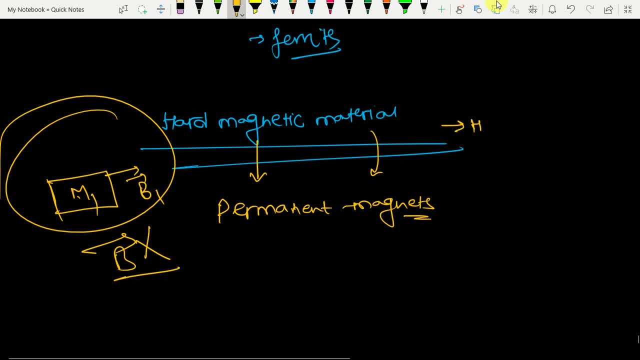 retentivity will be more. what is the properties of hard magnetic? what is the properties of hard magnetic? what is the properties of hard magnetic materials? so you can say that high materials, so you can say that high materials, so you can say that high retentivity. 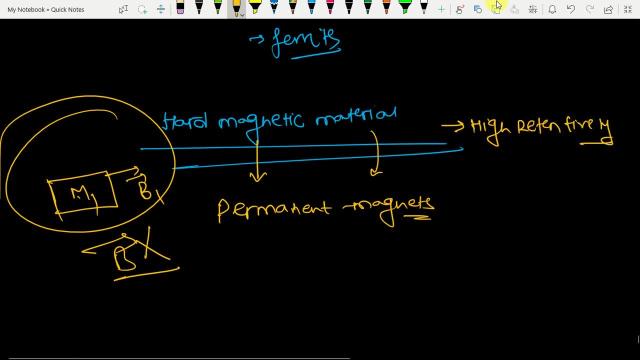 i have explained retentivity in my. i have explained retentivity in my. i have explained retentivity in my hysteresis log loop concept. i will hysteresis log loop concept. i will hysteresis log loop concept. i will explain again, don't worry. 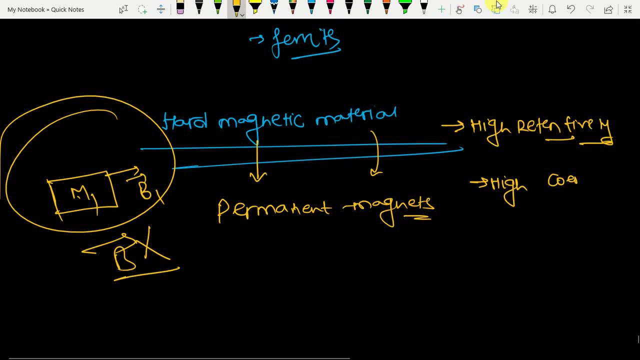 explain again, don't worry. explain again, don't worry. high coercive, high coercive, high coercive cohesivity, cohesivity, it is a negative magnetic cohesivity. it is a negative magnetic cohesivity, it is a negative magnetic intensity, which which we have to apply. 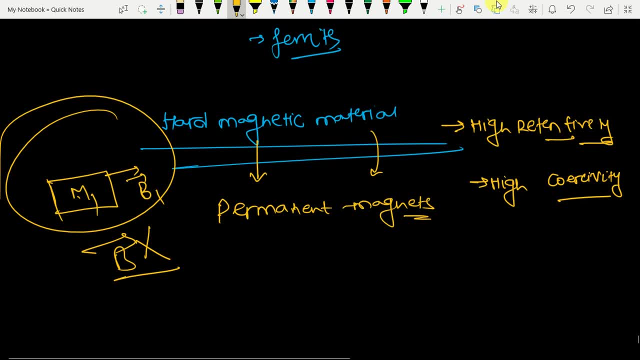 intensity which which we have to apply, intensity which which we have to apply so that the residual magnetism, so that the residual magnetism, so that the residual magnetism of that material will remain, will equals of that material will remain, will equals of that material will remain, will equals to zero up cassidy hc code zero. 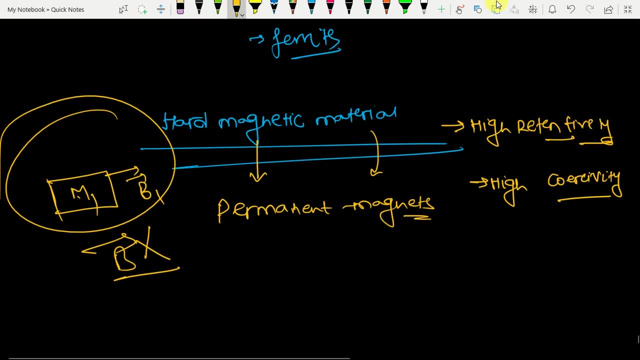 to zero up cassidy hc code zero. to zero up cassidy hc code zero, so that the remain residual magnetism, so that the remain residual magnetism, so that the remain residual magnetism will be zero. i will explain, i am going will be zero. i will explain, i am going. 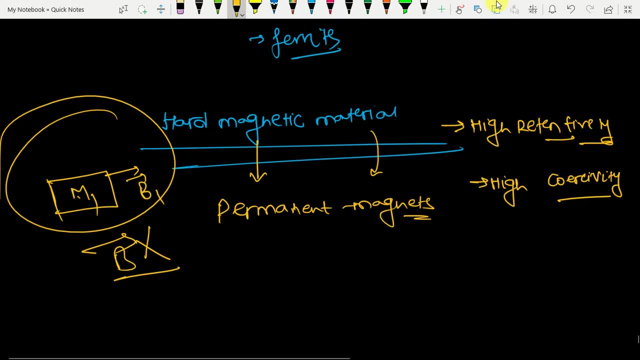 will be zero. i will explain. i am going to draw again bh curve so that you will to draw again bh curve, so that you will to draw again bh curve, so that you will be able to understand it easily. if you be able to understand it easily, if you. 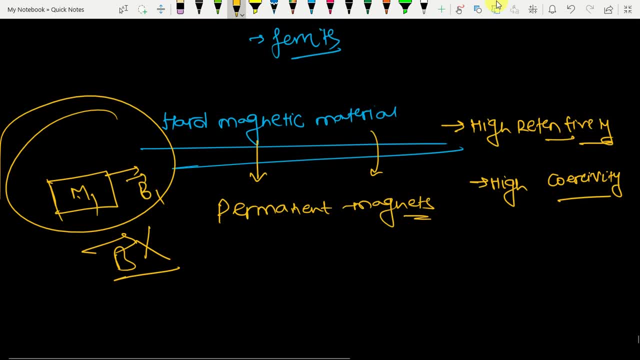 be able to understand it easily. if you haven't referred my previous in, haven't referred my previous in, haven't referred my previous in previous lecture, lecture number 20. you can. previous lecture, lecture number 20. you can. previous lecture, lecture number 20. you can refer it for bh curve analysis now. 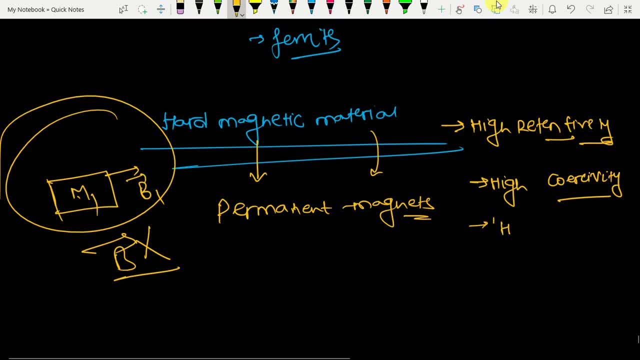 refer it for bh curve analysis now. refer it for bh curve analysis now. in case of hard magnetic material. in case of hard magnetic material, in case of hard magnetic material, hysteresis loss, that is, ph, will be high. hysteresis loss, that is, ph, will be high. 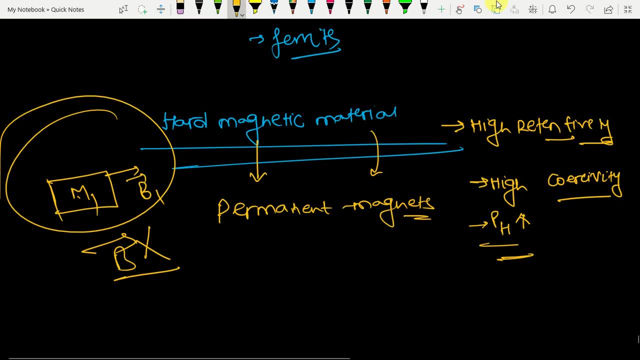 hysteresis loss, that is, ph, will be high. why q high hysteresis loss? because why q high hysteresis loss? because, why q high hysteresis loss? because for hard magnetic magnetic material, the. for hard magnetic magnetic material, the. for hard magnetic magnetic material, the bh loop is wider. 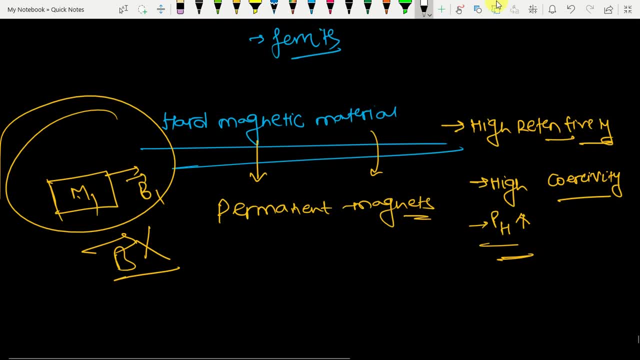 bh loop is wider. bh loop is wider. that's why it have high hysteresis losses. that's why it have high hysteresis losses. that's why it have high hysteresis losses. so it's very simple now. so it's very simple now. 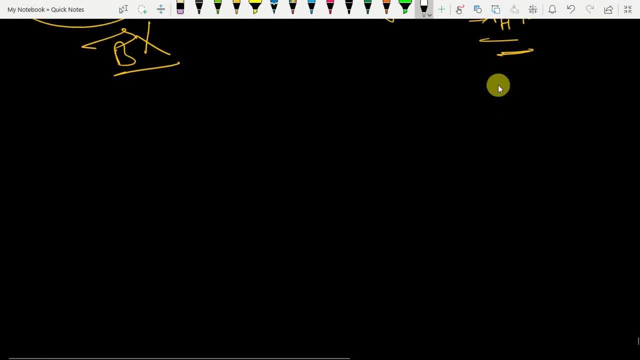 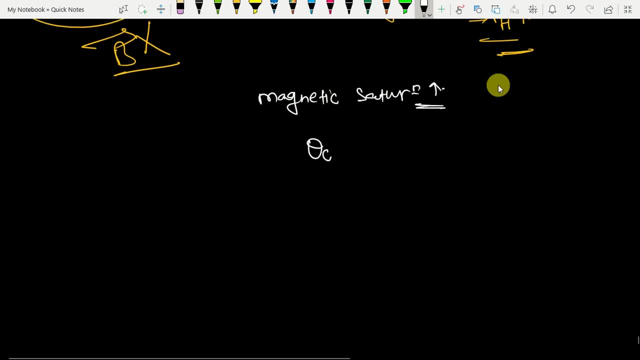 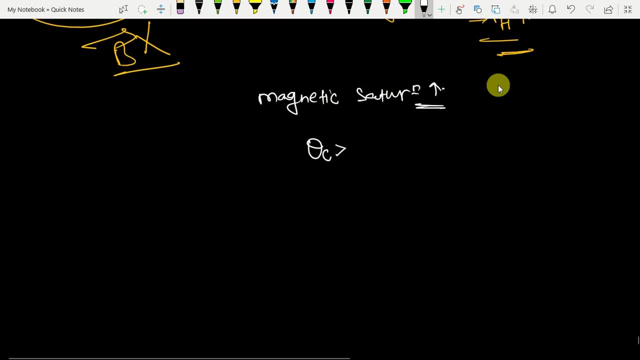 material ever is a jada honey. material ever is a jada honey. what ferromagnetic material up me? what ferromagnetic material up me? what ferromagnetic material up me? existence code idea to yet you curie. existence code idea to yet you curie. 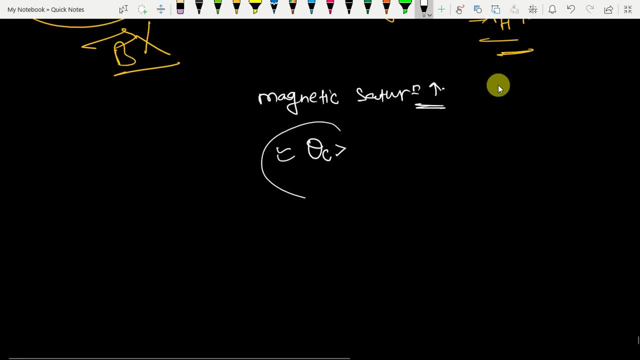 existence code idea to yet you curie. temperature is key. I okay, this is the temperature is key. I okay, this is the temperature is key. I okay, this is the only advantage of using ferromagnetic, only advantage of using ferromagnetic, only advantage of using ferromagnetic material or hard magnetic material. 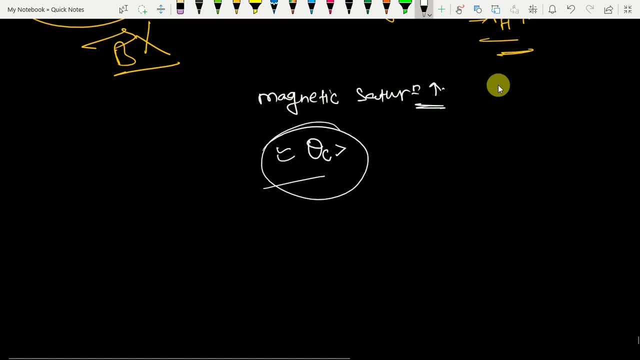 material or hard magnetic material. material or hard magnetic material because its curie temperature will be high, because its curie temperature will be high, because its curie temperature will be high in case of hard magnetic material P, in case of hard magnetic material P, in case of hard magnetic material P into H, max, jada that is, it will be more. 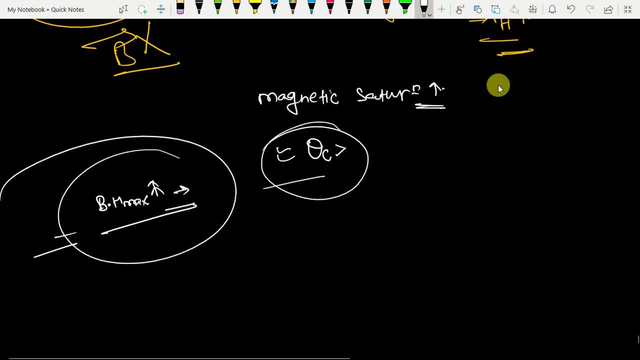 into H max- jada, that is, it will be more. into H max- jada, that is, it will be more. in case of hard magnetic material. you, in case of hard magnetic material, you in case of hard magnetic material. you can remember this. now let me draw BH. 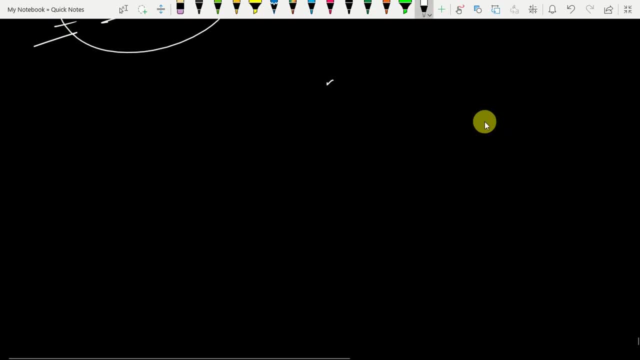 can remember this now. let me draw BH. can remember this now. let me draw BH curve of both soft magnetic material and curve of both soft magnetic material and curve of both soft magnetic material and hard magnetic material and justify hard magnetic material and justify hard magnetic material and justify through this diagram. let's draw for hard. 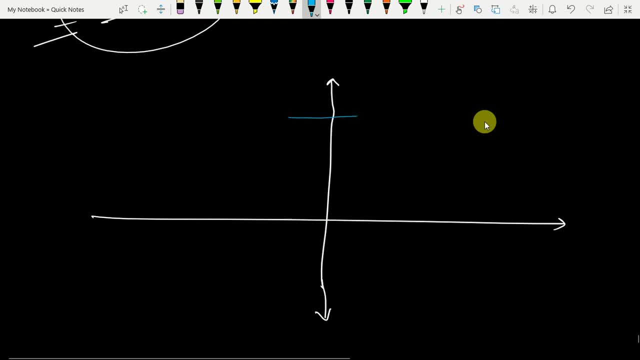 through this diagram. let's draw for hard through this diagram. let's draw for hard first. let's say like this: I am first. let's say like this: I am first. let's say like this: I am trying just casual. you know I don't want to, trying just casual, you know I don't want to. 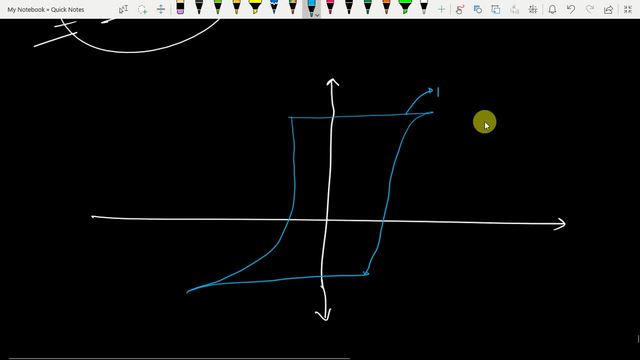 trying just casual. you know, I don't want to draw like a. this is for hard magnetic draw like a. this is for hard magnetic draw like a. this is for hard magnetic material. now let's draw for soft material. now let's draw for soft material. now let's draw for soft magnetic material. 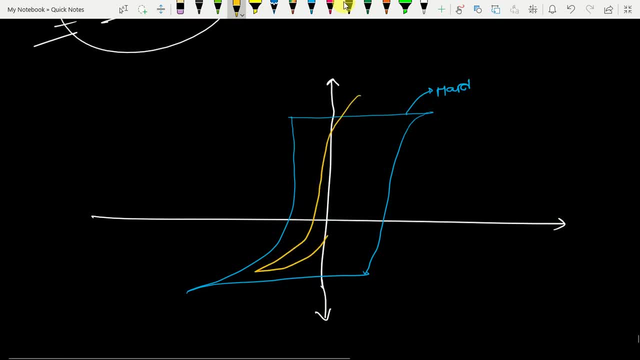 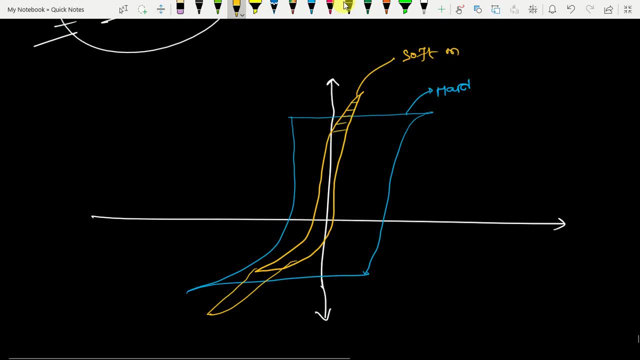 magnetic material. this is a approximate curve. I haven't draw it like perfection curve. I haven't draw it like perfection curve. I haven't draw it like perfection, but it is approximate curve you can. but it is approximate curve, you can, but it is approximate curve. you can understand that the looper, the wider. 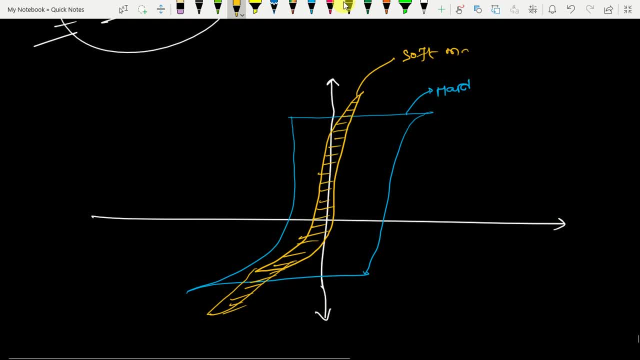 understand that the looper the wider. understand that the looper, the wider area. the loop area is a small. in case of area, the loop area is a small in case of area. the loop area is a small in case of soft magnetic material- soft magnetic. soft magnetic material- soft magnetic. 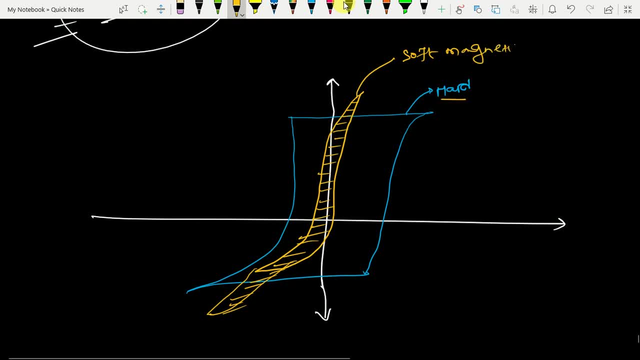 soft magnetic material. soft magnetic material. this one is hard magnetic material. this one is hard magnetic material. this one is hard magnetic. materials in soft magnetic material. this materials in soft magnetic material. this is the saturation point bs. saturation is the saturation point bs. saturation is the saturation point bs. saturation saturating magnetic field for hard. 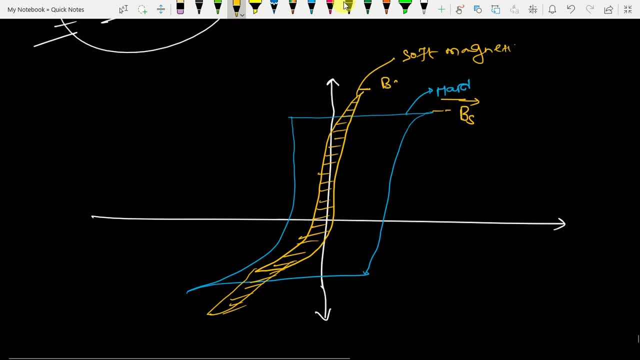 saturating magnetic field for hard saturating magnetic field for hard magnetic material. and this is a magnetic material and this is a magnetic material and this is a saturation magnetic field for soft saturation magnetic field for soft saturation magnetic field for soft magnetic material. now you can say that 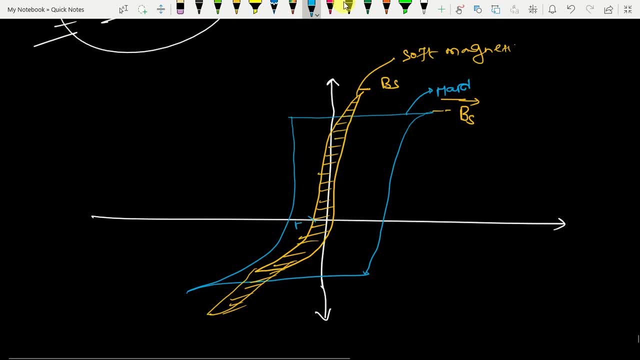 magnetic material. now you can say that magnetic material, now you can say that let's take, this is the let's take, this is the let's take. this is the coercive hc, that is coercive effect for coercive hc, that is coercive effect for coercive hc, that is coercive effect for soft magnetic material, and this is the. 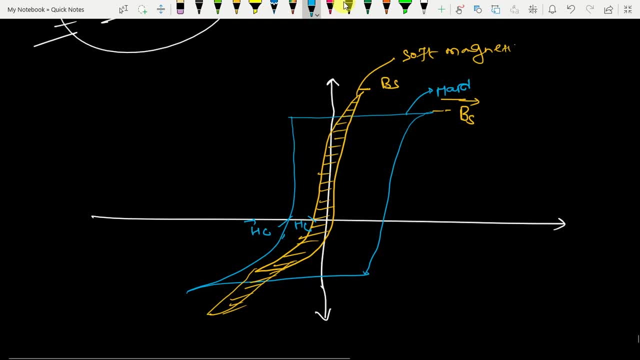 soft magnetic material and this is the soft magnetic material and this is the coercive effect for coercive effect for hard magnetic field. coercivity, that is the force required to draw the magnetic field, to reduce the internal residual magnetic field inside a crystal, that which we have already exposed inside a 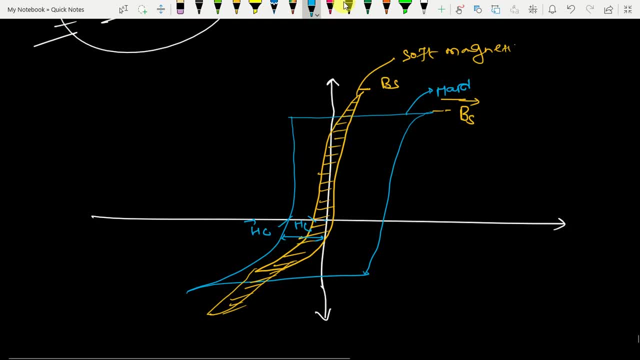 magnetic field is zero, is high in case of harder material or hard magnetic material, and this is software. so you can see that as the loop area is less, losses will be less. that's why we we prefer soft magnetic material in case of making transformer core or or any core of ac. 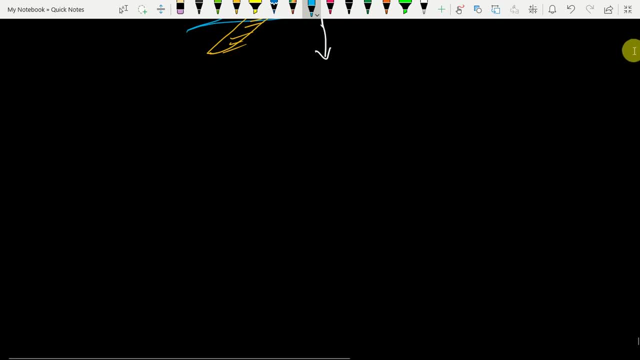 alternating machine and all now there are some of the hard. example of some hard magnetic materials are carbon steel. carbon steel is used in as magnetic latch relation and compass needle, compass needle tungsten steel. it is used as a magnet in case of dc motor. permanent magnet in case of dc motor. 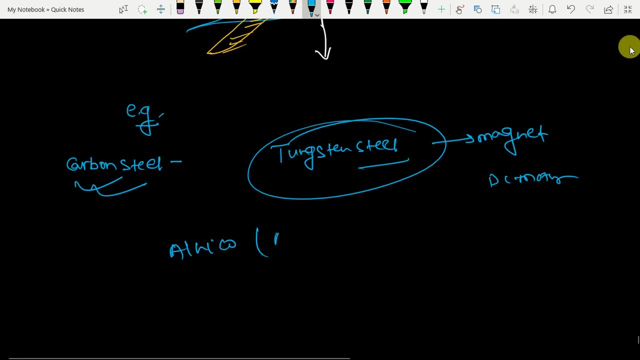 alnico, it's an alloy containing aluminum, nickel plus cobalt. remember these things you can expect. question, a direct question, you can ups, you can frame from this, so you don't have to left anything, anything out of that. ELNICO: it's magnetic property is stable with time and temperature. 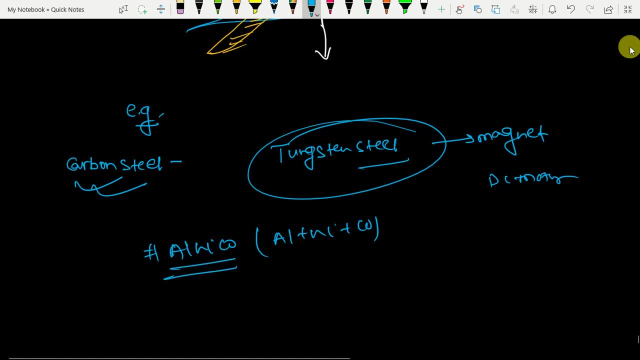 we are using ELNICO because its magnetic properties are stable as it is if we will vary the temperature and as well as time. they are stabilizing the magnetic properties when that is rather stable than iron, orvak iron and coolisc respectable the magnet of nickel. this isあっ оперative heat, MPH. magnetic properties are stable with time and temperature. we are using all nickel because it's magnetic properties are stable, as Bl relying álico has. magnetic properties are stable as Liko If we will vary the temperature and as well as time. they are stable. they are stable with the temperature and as well as time. they are stable when we sold is associated with time and temperature. 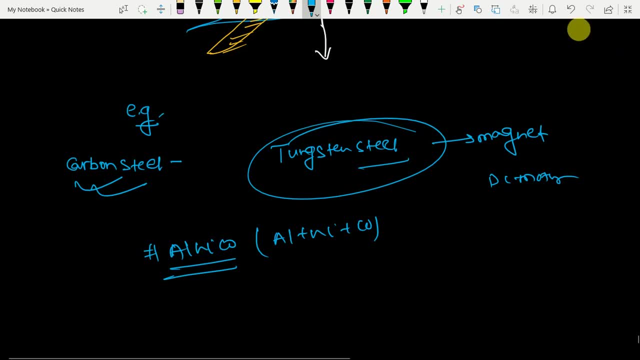 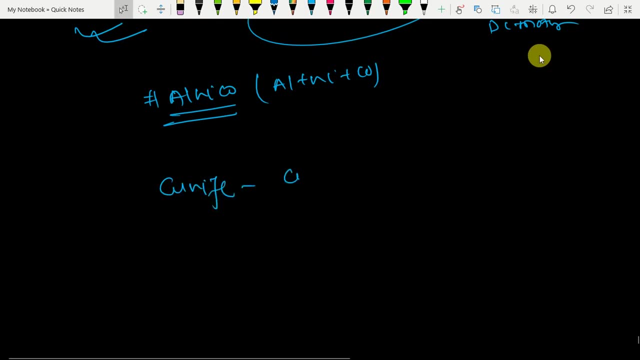 temperature and as well as time. their stability, that is, BH curve, will remain stable up to certain range of temperature. cuneify, that is copper, nickel and iron. this is the alloy of these three and example our Fahad is also chromium steel. now, these things you have to know about soft and hard magnetic. 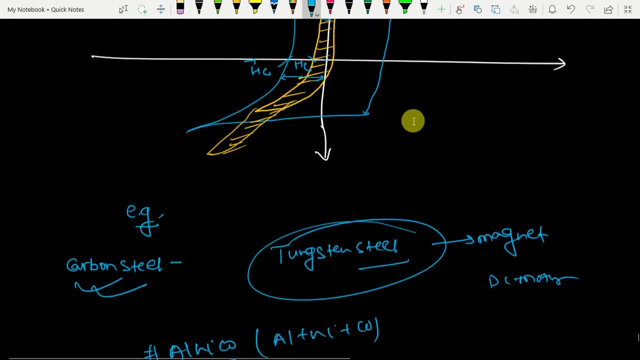 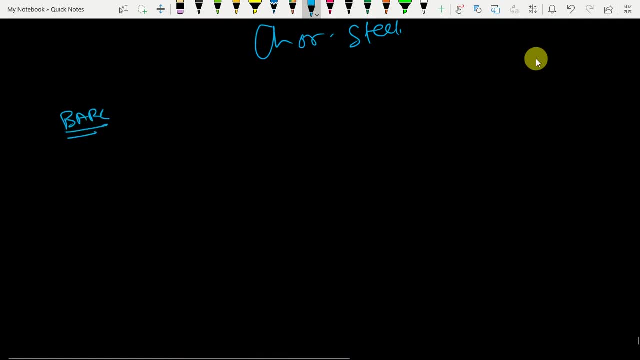 material. now let me explain you a few question that they can ask in interview, that is, you can expect question related to these in BRC and many exams- why we are not able to add that this one of a small amount of silicon to software and improves many quantities, that is, if other I'm add, got them on low, if you. 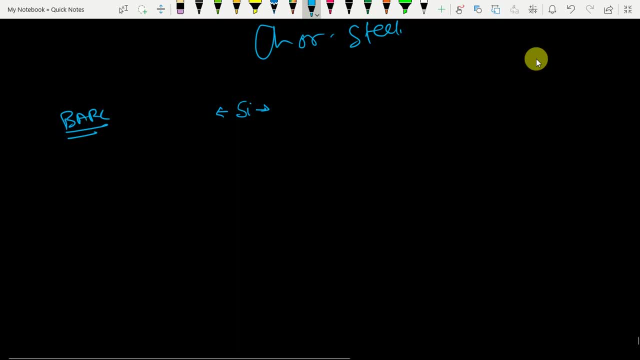 will add some small amount of silicon to any fairer, any magnetic material. that is ferromagnetic material. what sorry? quality is improved and that is, resistivity of that material improves, go easy. force, that is HF or HC, you can say it reduces, that is there. there will be required some negative magnetization. 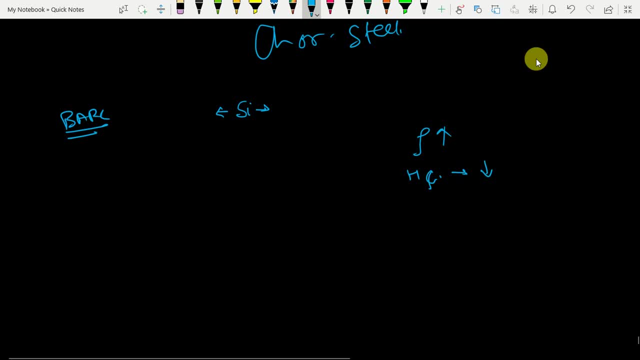 less magnetic, negative magnetization, so that we have to remove the residual magnetism of that a specimen which is placed, which was placed inside a magnetic field, stability increases, stability of magnetic characteristic improves. that is, if you will add some silicon, silicon care, decent say, Cassidy- ferromagnetic material, may oski resistivity will. 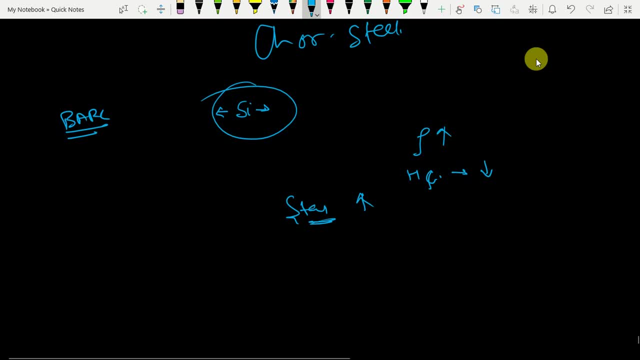 increase, not letů 1 to you 14 in India, in India thisultura, and really he was 1, if you will add 2 or 3, anschütаются emult every single material. the resistivity will increase 4 times 10's Coloradoclub in Iran: small iron wirdərестivity. si meera 기 flavored medical records 14 times every time. urban o 30 ca non antika grafters. id nay gra Criminal rend則. 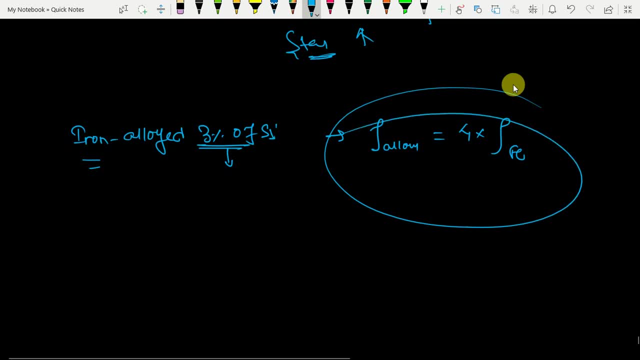 times say normal iron key. comparatively that is 10% silicon add key. I have added only 3% of silicon. it has improved four times of resistivity. you can, you can expect or you can imagine the effect of resistivity on any material. you can say that now normally we are allowed. 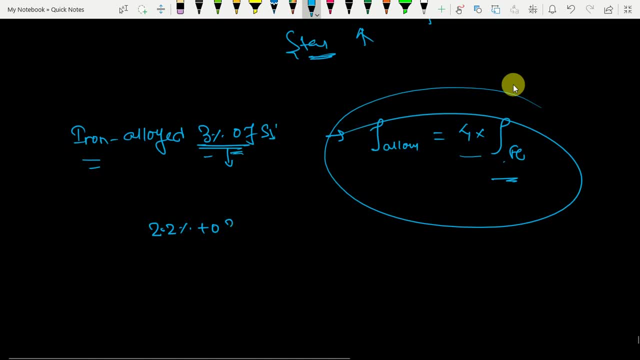 to add 2.2% to 3.4% of silicon. addition is about 5% of maximum. addition of 5% is allowed in case of iron silicon. 5% of silicon is maximum capability of an iron. if we will add silicon, 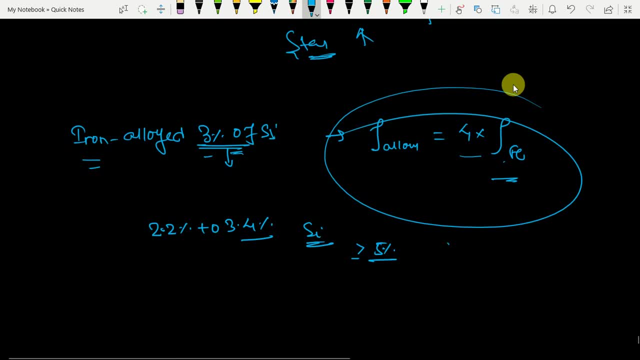 more than 5% in case of an iron, the iron will be become brittle and we will have some difficulty in working with. so there are some boundary relation that we have to keep it less than 5%. the second, the last question, or second last question you can expect, is that choosing? 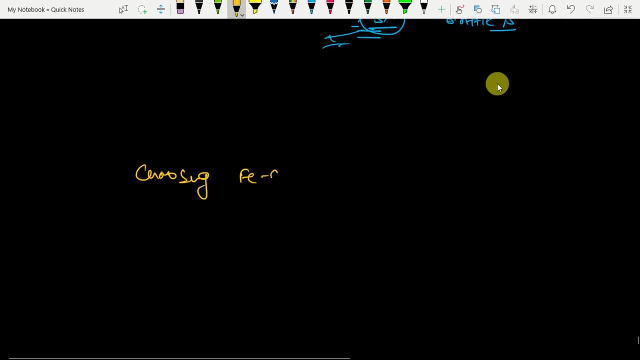 iron- silicon alloy for transformer core. a question will be asked why we have we are choosing iron- silicon alloy for transformer core- transformer core. then you will say that core of transformer is soft magnetic materials. to minimize hysteresis losses, the steel used for transformer cores may be hot rolled and 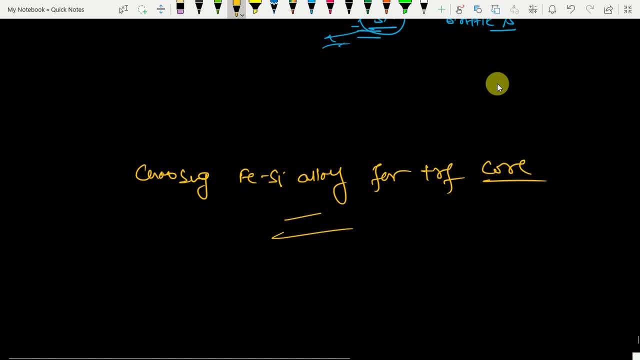 cold rolled. you can say that. now I'm talking last topic. I'm talking about three-phase induction motor, induction machine. this motor is used in most widely using motor in the steel application. you can say that core of transformer is soft magnetic materials to minimize hysteresis losses.